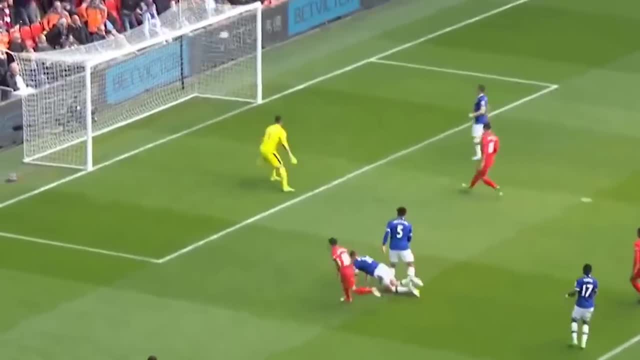 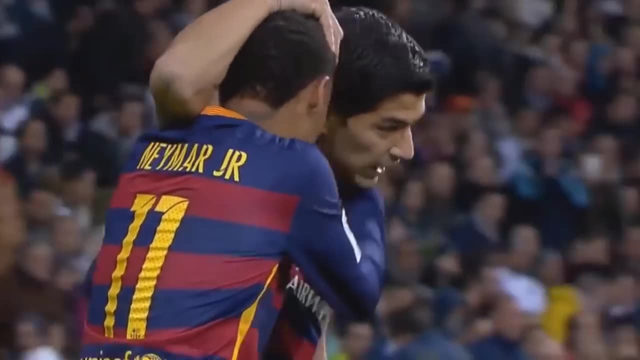 where one time you just focus on your position and then you analyze the game. Another match where it's everything. but for the most part I find that analyzing the player just playing in my position is more effective. So another good thing you can do is actually get out a pen and paper or pad and pen and write down some. 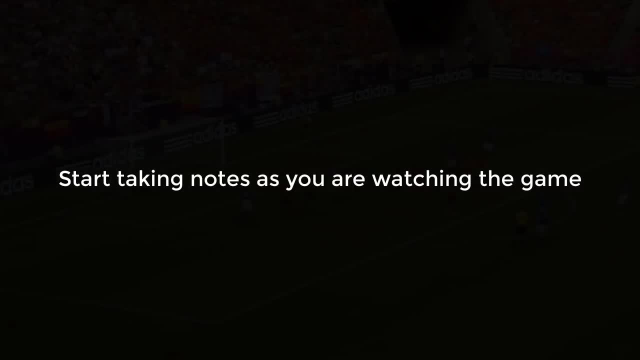 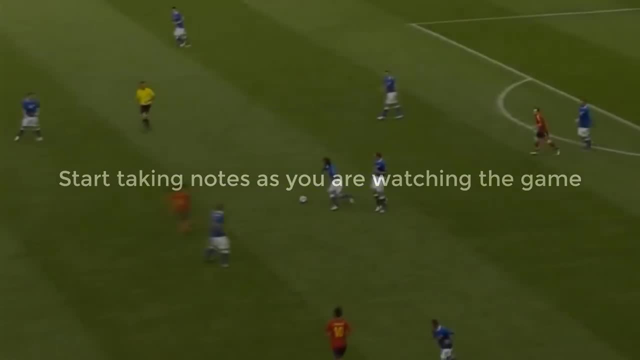 things while you're watching the player. Now you want to look out for certain things and have some certain questions on your mind as things are happening. You want to be continually analyzing each play that your players involved in to see what you should be applying to your own game. So, for example, if I'm watching 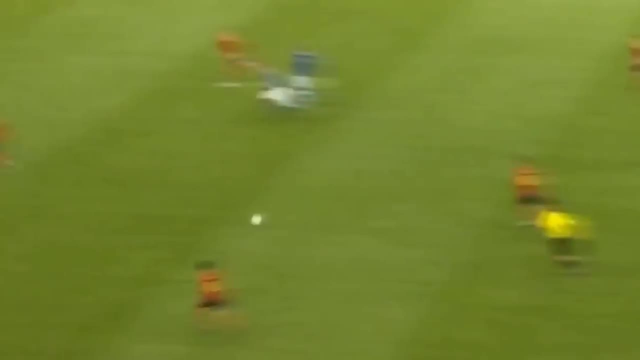 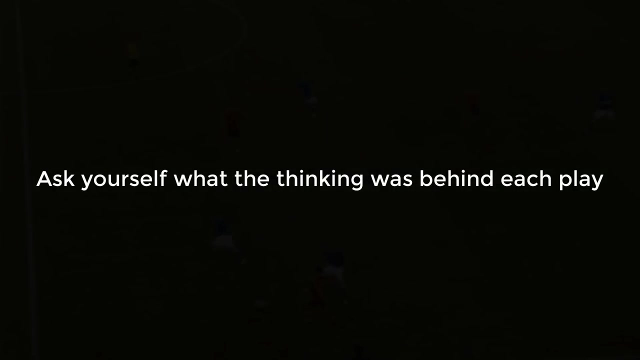 Harry Kane play and he makes a certain run. I want to be asking myself: why did he make that run? What was the the point of making that run? Obviously he had a plan in mind. what actually happened, and what did he plan on happening, If for 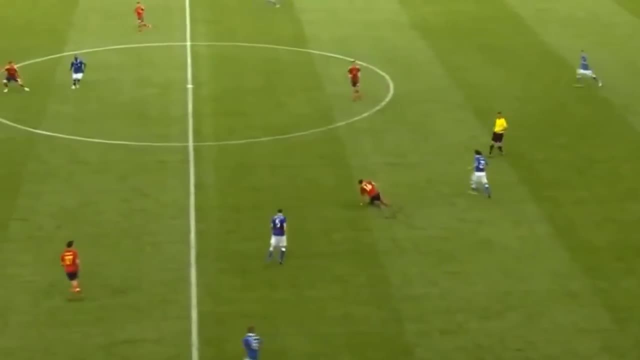 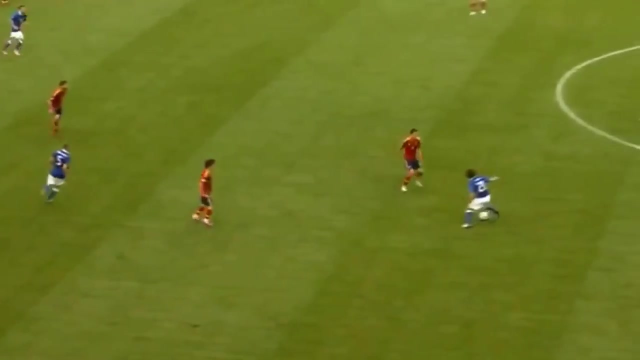 example, your player doesn't move, or to opened up space or something, or makes a good decision. why did he do that? You know, ask yourself these questions because when you come to the answers, you'll realize: oh, I should be focusing on these things as well. Maybe, for example, he picked out one. 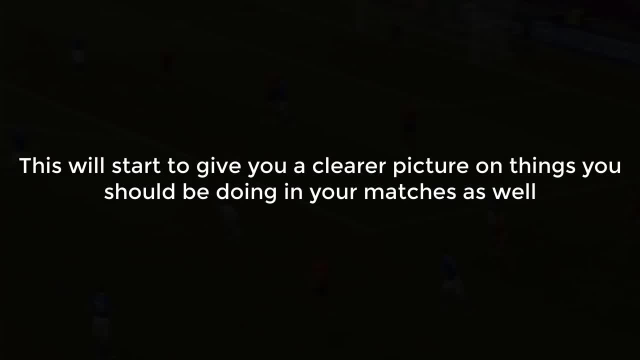 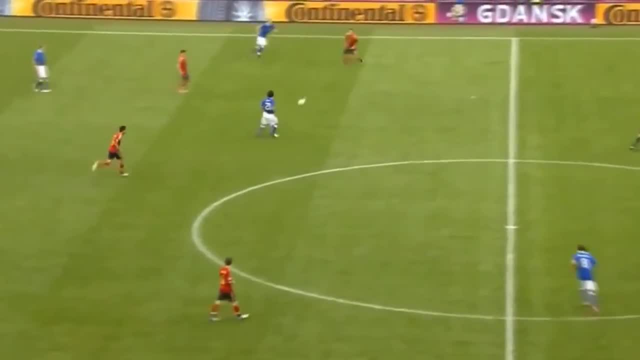 pass instead of another really obvious pass and you have to ask yourself: why did he do that? You can even pick up on the mistakes of the players you're watching. So again, if we're using Harry Kane as an example- and I'm watching him and he makes a mistake, I can go okay. why did that mistake happen? What could? 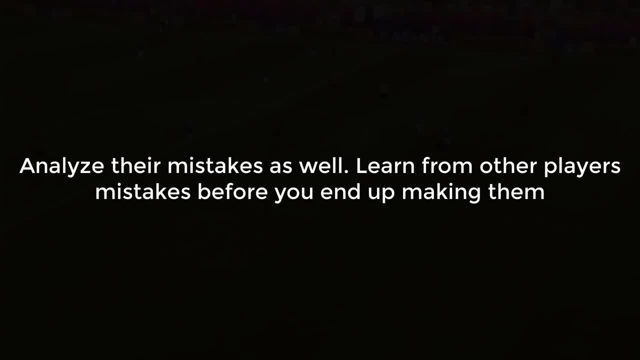 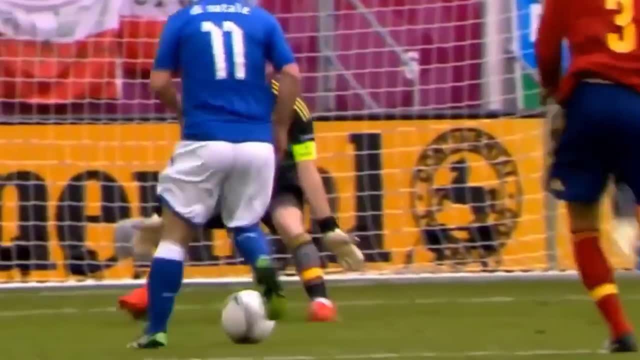 he have done instead in order to not make that mistake. That's very important as well. you can learn from the mistakes of others. In fact, it's a great thing to do so that you don't make those mistakes when you go into your match. OK, and I? 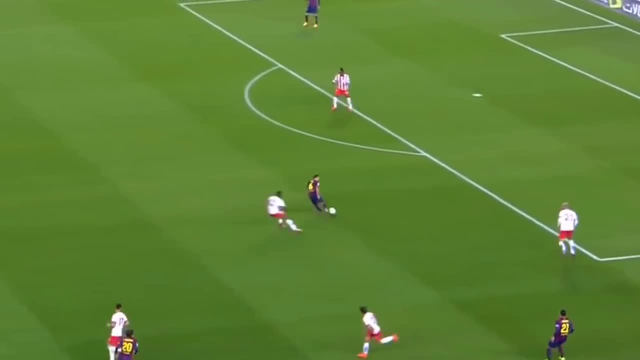 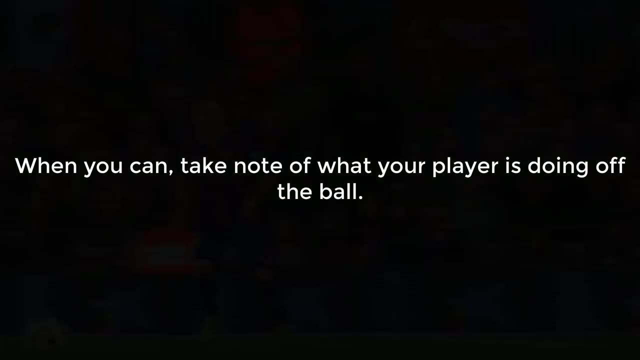 already mentioned this briefly, but you want to see what the player is doing off the ball. now, i understand that sometimes, for certain positions, the camera will not be on them, so you kind of have to do this as well as you possibly can, but for whenever the player you're analyzing is on the pitch, watch him. 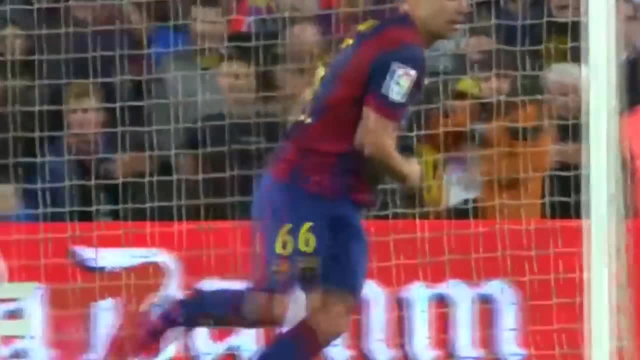 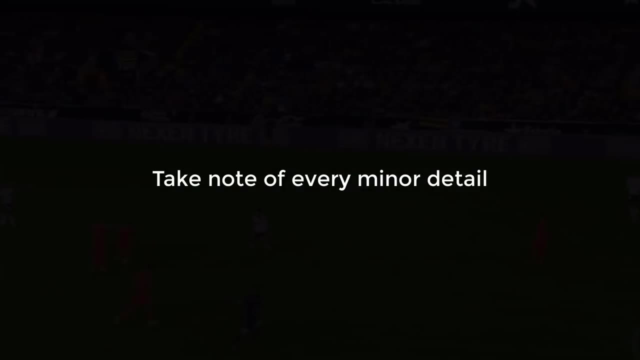 watch what he does. does he make certain runs? does he kind of start walking and burst into space? what positions does he take up? you know, what does he do with the ball when he has it. what does he do when he doesn't have the ball? how does he make himself available for the ball? how does he open? 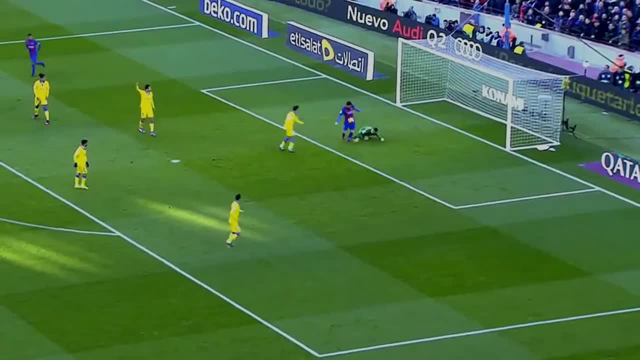 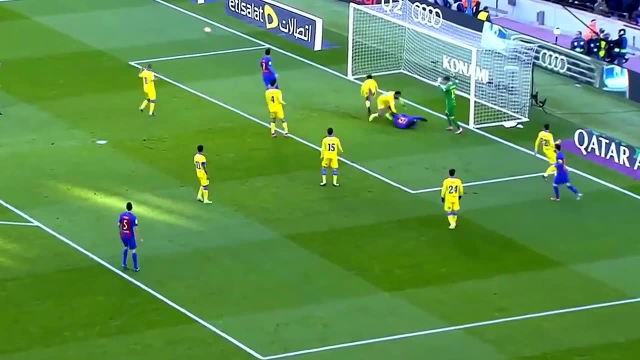 up space with different runs and movement for his teammates by the end of the match. i want you to pretty much answer a few questions about the performance of your player now. um, let's consider that they had a good match. i want you to ask what were some of the common things or things they did. 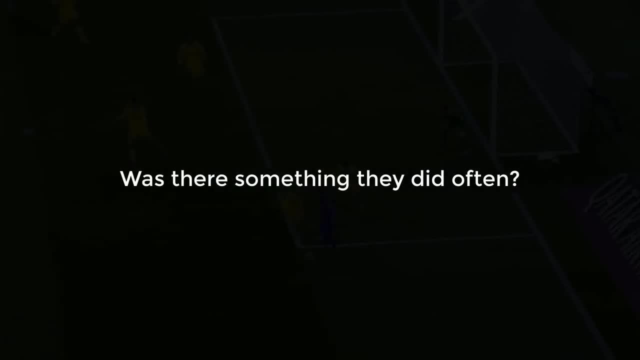 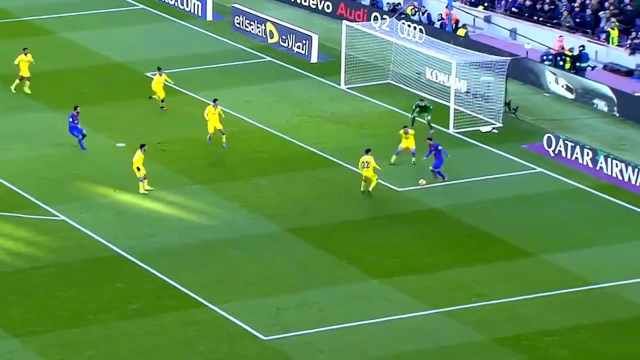 over and over again, consistently. so was there a common theme among their play? um? so, for example, were they shooting a lot? were they doing a certain move a lot? did you notice, for example, um, if you're watching suarez, you may have noticed that he uses the chop move a lot. that's something to note. 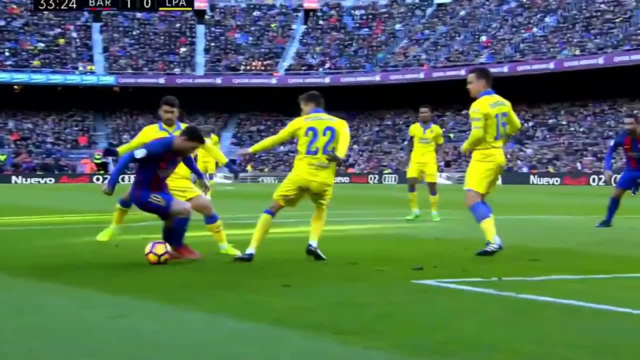 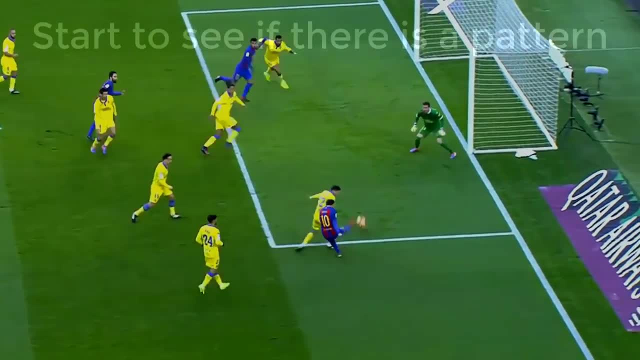 because there's a reason he's doing it more than once. is there a certain run being used more than once? is there some space that they occupy more than once? is there a certain play they try and do more than once? once you start picking up on these patterns, you can start trying to figure out. 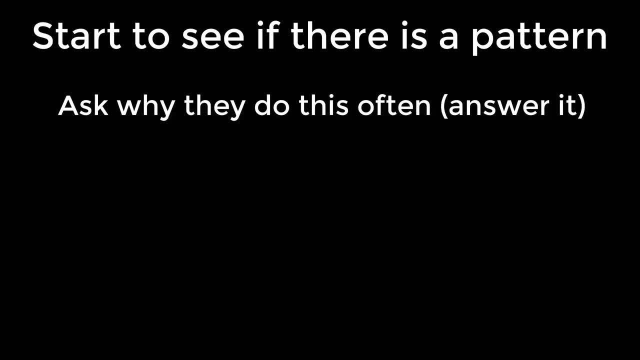 why these are going on. why are they doing these specific things that you're writing down and you've observed over and, over and over again? because this is by design. there's a reason, they're doing it more than once and you're trying to figure out why these are going on. 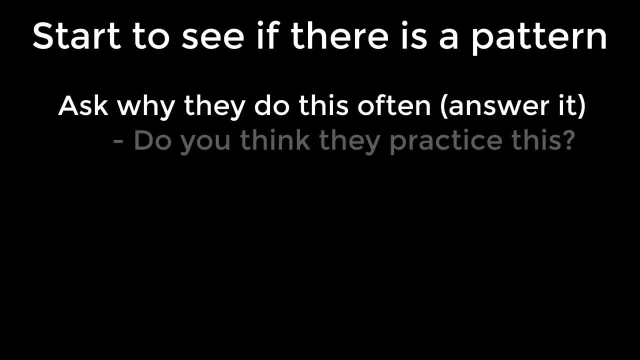 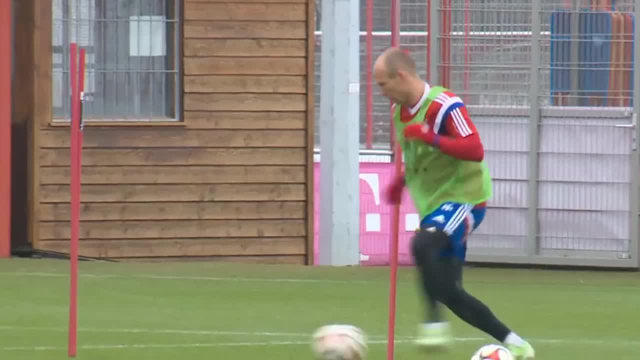 certain things over and over again, and one of the probably most likely reasons is they're practicing these things over and over again in training so that they can do them consistently in matches. so that's something to take into account. what are the common themes? what is the? 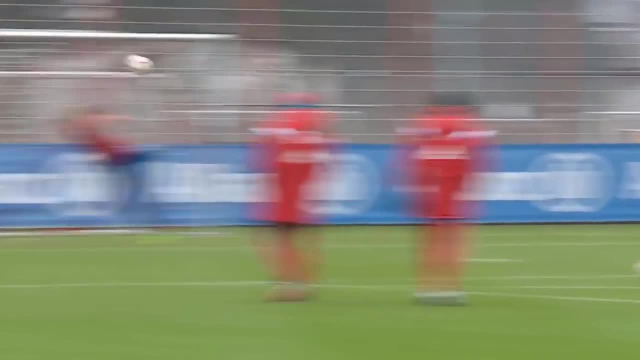 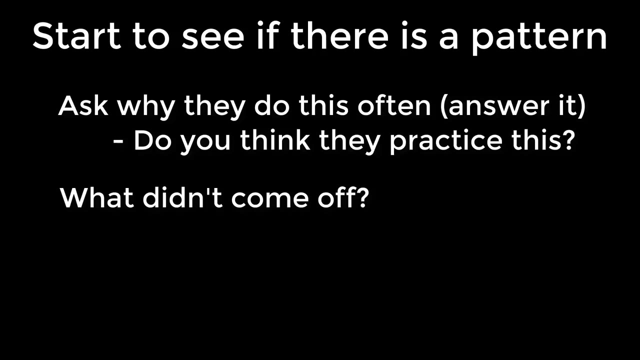 player you're analyzing doing very often. another thing to consider is what did not work for them. what is something they didn't do that often, but when they did try, it didn't work. now this doesn't necessarily mean you won't be doing these things. it could just be it didn't come off, but it's still. 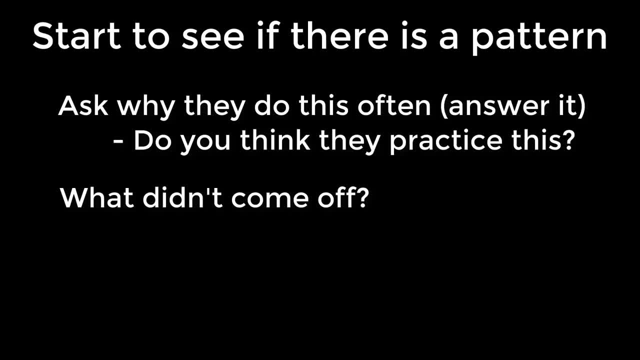 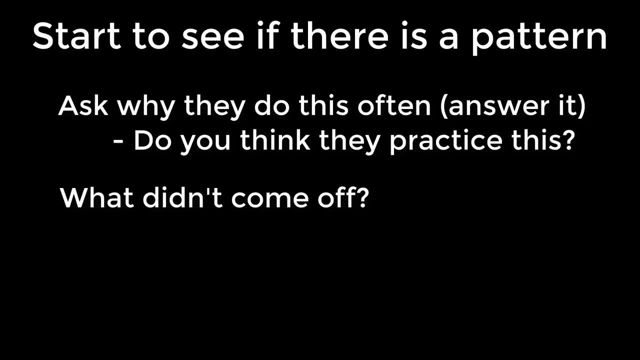 again: um, we're opposed to um 25 yards or closer, he shot and it was very effective. um, you know, there was a certain run he kept making that was never- you know, never- got him the ball, but there was another run he was making which got him the ball. often, you know making these comparisons. 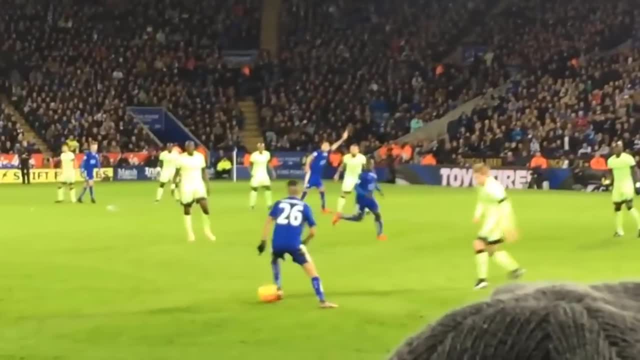 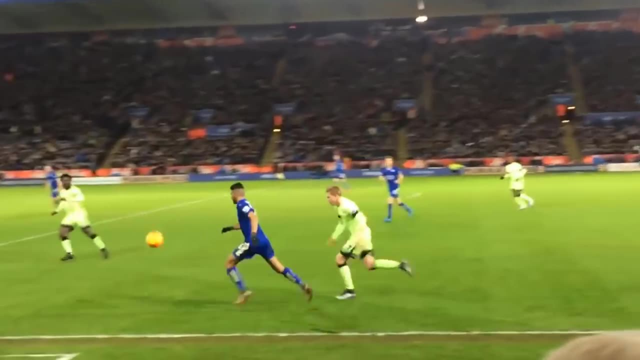 will um kind of it'll seep into your mind and you'll start to recognize these patterns when you're in matches as well. so you don't only want to identify what it is he was doing often that worked. identify what it is he was doing often that worked. identify what it is he was doing. 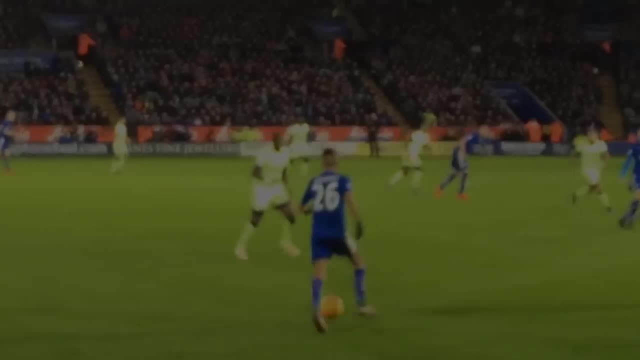 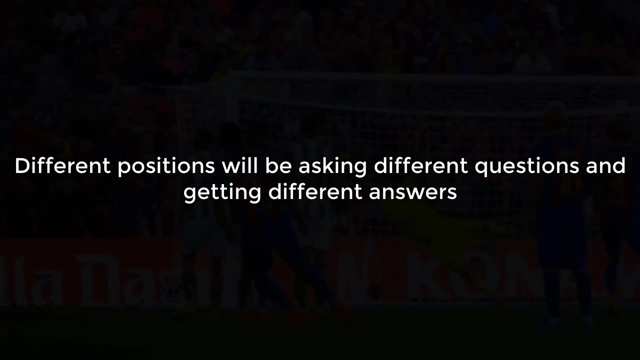 what he was doing. that wasn't working. now, some of these will also be specific per position, for example, defensive positions. you'll be asking different questions than attacking positions, for example, if i'm, i'm attacking player, so if i was watching a certain player, i would ask things. 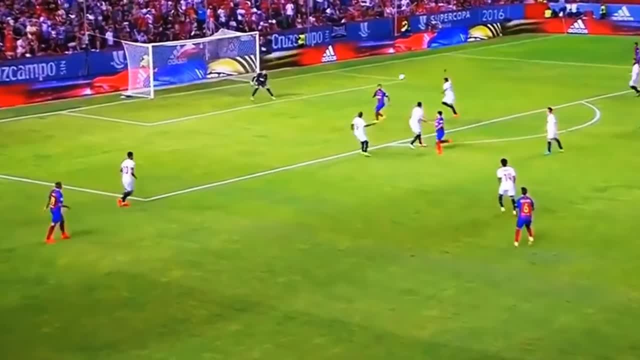 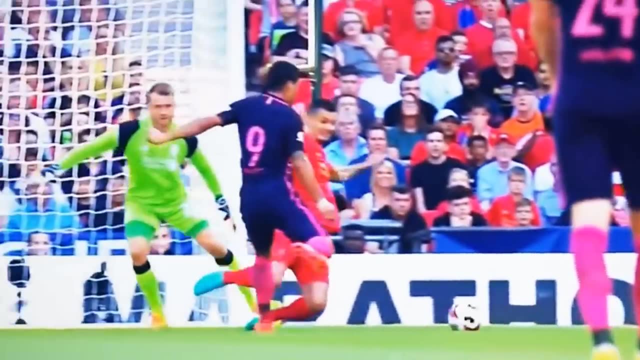 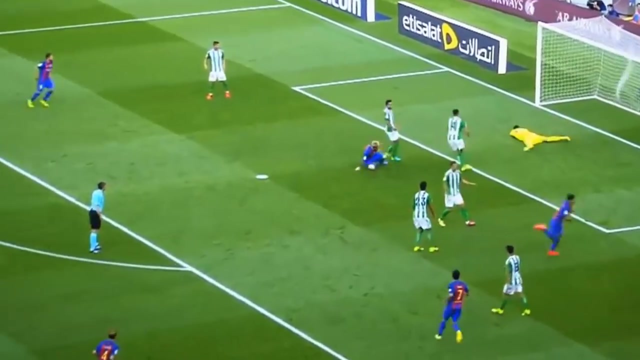 like: what skill moves is the player using often and when is he using them? that's a good question to ask. again, like i mentioned, what runs is the player making and when is he making them? i would ask: when does he seem to check to the ball? um, when does he seem to make this certain play? when does 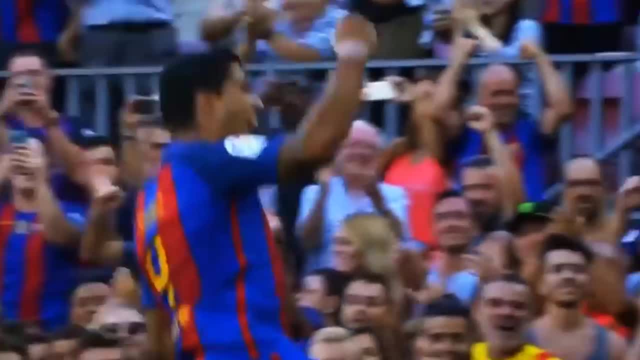 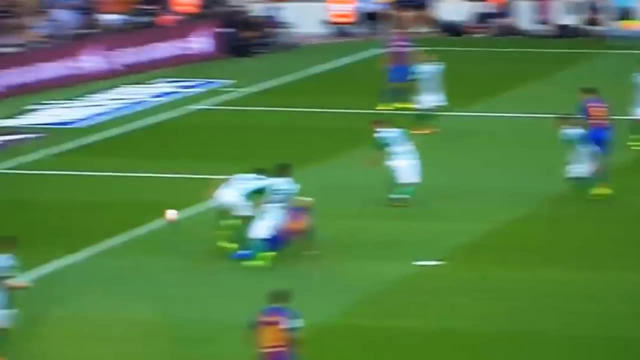 he seem to move into this space, and why does he move into that space? if you're asking yourself these things and then answering these questions, you'll start to recognize why they're doing these things and again, then you can apply it to your own match, okay. and after you've done that, you've 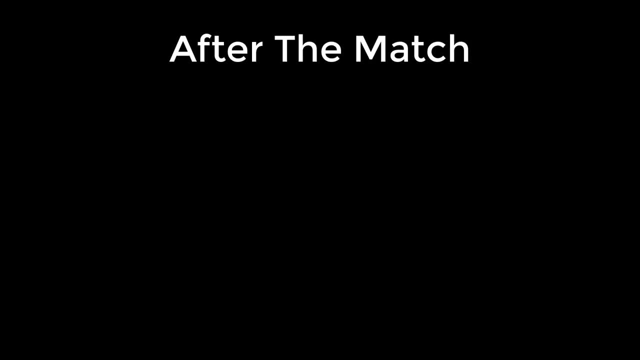 basically analyzed the performance of the player, what was working, what wasn't- you can pretty much write down. what can i apply to my own game? remember, the whole point of analyzing these matches is to get something out of it that will be applicable to your own game. of course, watching these will. 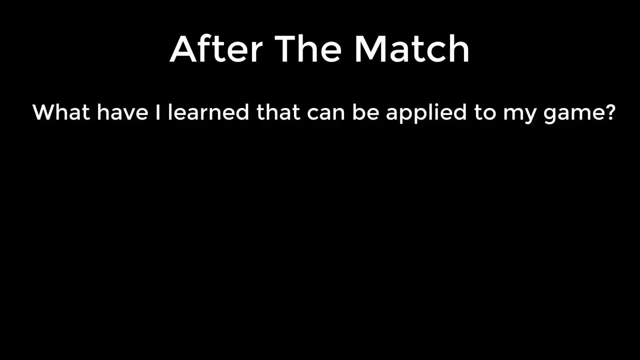 also improve your soccer iq, which will be applicable to your own game. but you don't want to just analyze the player and then not relate it to yourself. so once you've analyzed everything, then you go: okay, this is what it was, this is what happens. these are the patterns i'm seeing. 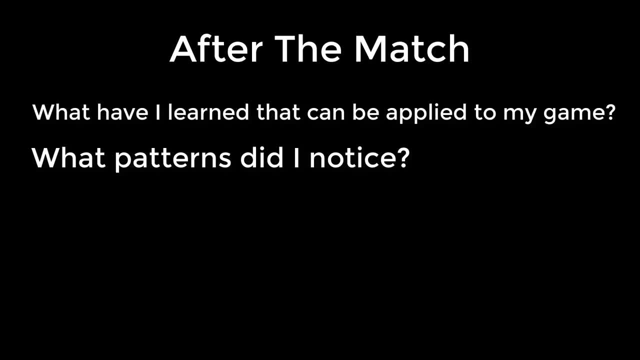 how can i apply this to my game? and then you can start making training sessions that maybe work on things you saw this player doing. often you can start to come up with ideas of things you can do in matches, things of this nature. so then you need to look at your own game and go. 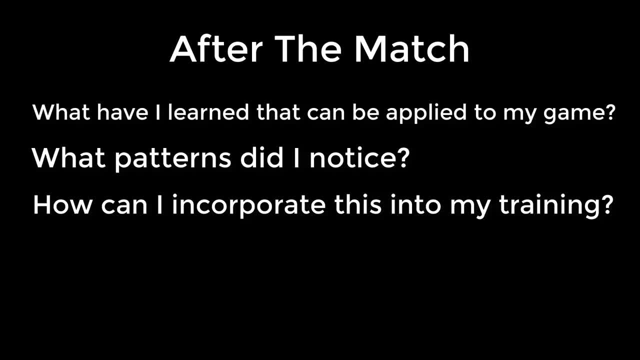 which things that i've identified and you'll start to see a pattern. after you analyze a few different matches or you watch a certain player over and over again that you're trying to emulate, you'll start to see a pattern of what you should be practicing, but that's when you need to start. 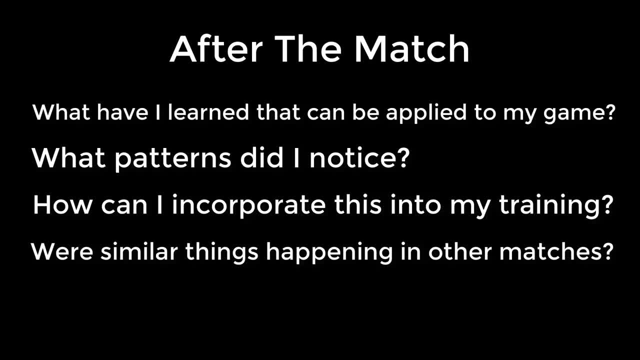 asking yourself: what should i be taking from their game and applying to my own? everything else you've done before that is useless if you don't apply it to your own game or don't relate it to your own game, because the whole point of analyzing these matches is to make you a better.